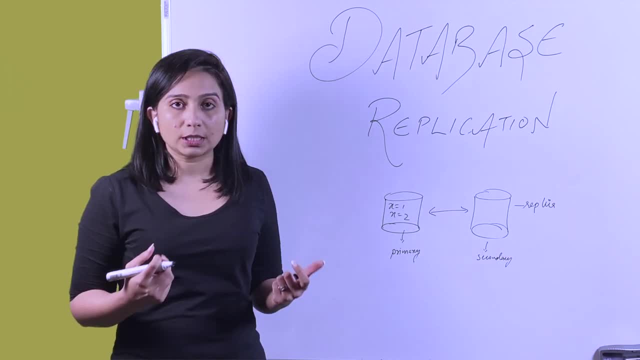 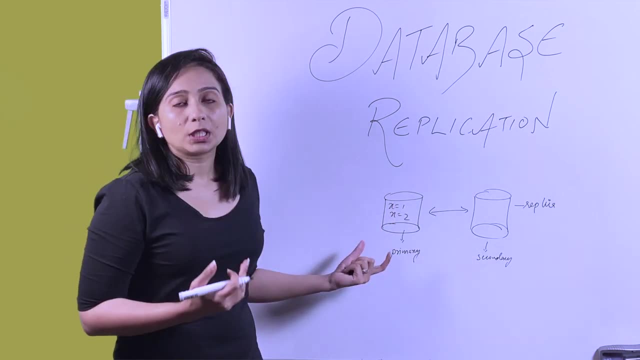 discussed fault and failure and we discussed fault tolerance. having a replica helps a great deal in tolerating faults. Let's say, for some reason the primary DB goes down or some network issue happens or something goes wrong with the hardware. 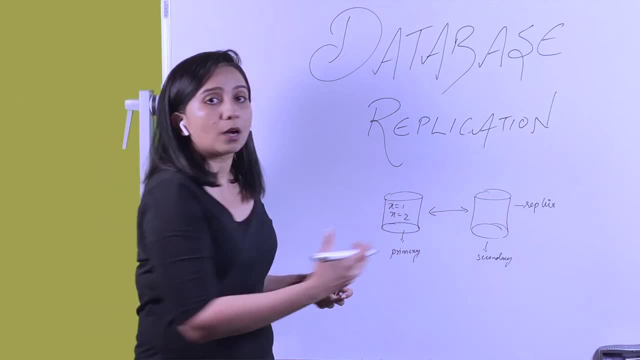 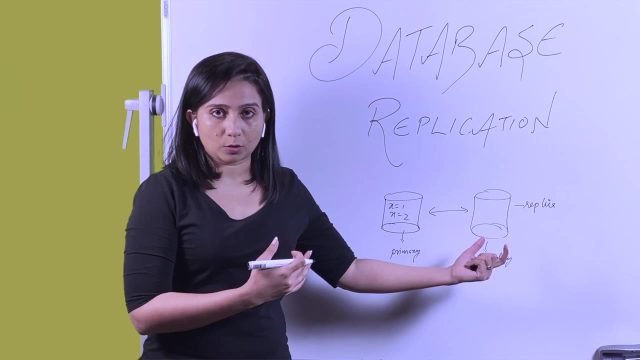 and we are not able to access the DB. In that case, having a replica helps. First, you would not lose the data, as you have your data replicated or copied onto some other location, And second, in some cases or in some implementations. 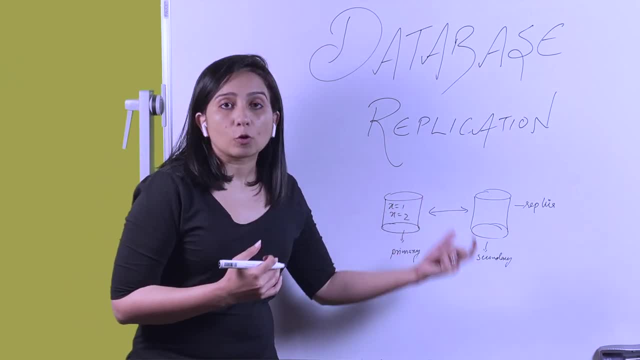 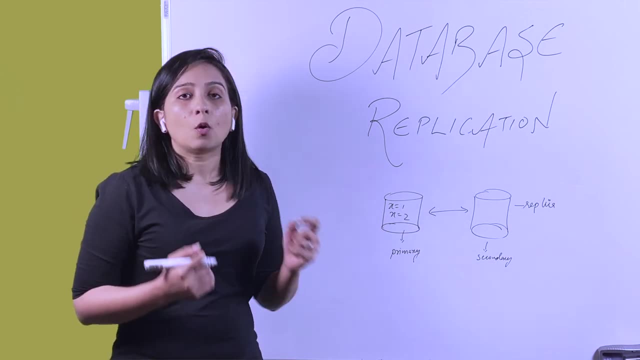 of different distributed DBs and systems. such replicas can also take over and become master DBs so as to save the system and the business overall. That is one primary reason, or one primary advantage of using replicas. Another advantage is, if you have seen the latency video. 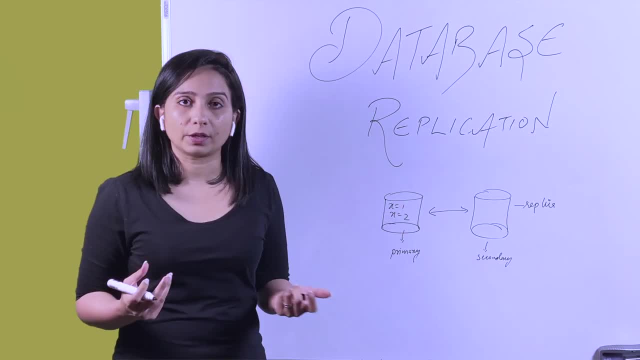 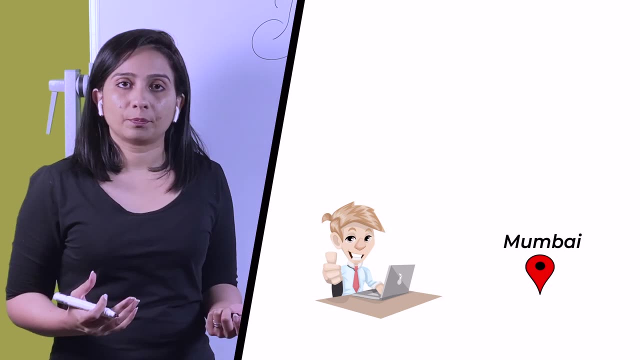 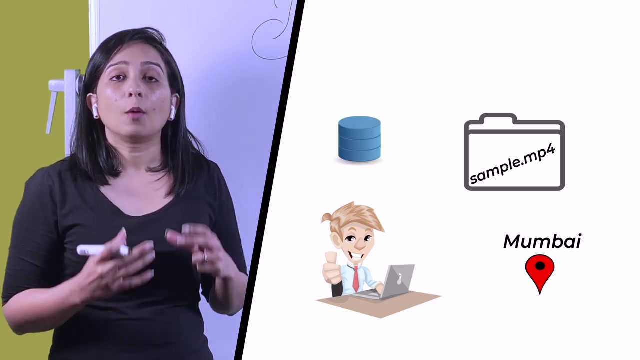 having replicas helps you reduce latencies. You must be wondering how or why. Think about this. You are watching this video. You might be watching this video from Mumbai, But the actual source video, the very first file or the primary video file, might be stored in some other data center. 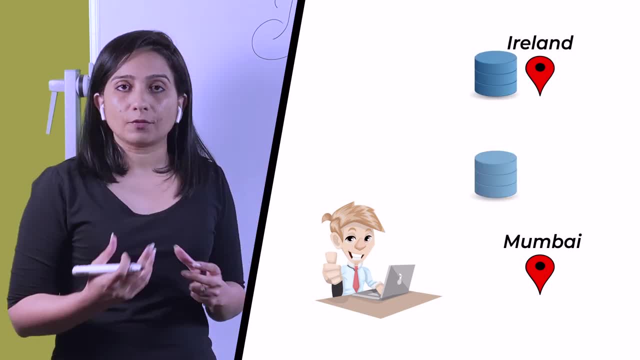 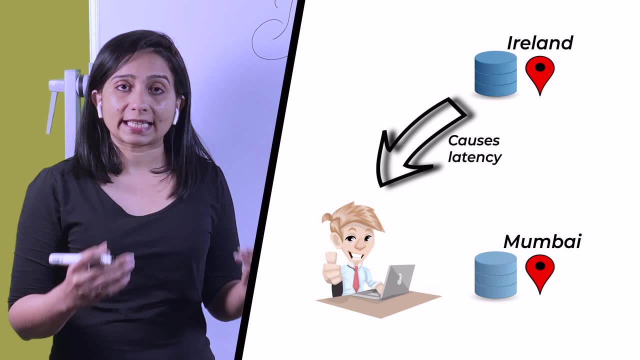 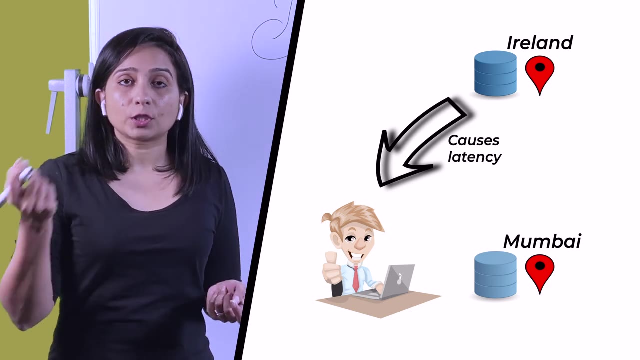 maybe I don't know- in Ireland, And the copy of that same video is available in Mumbai. Why? Because if you keep all the data at one place and it has to be accessed in geographically different or sparse locations, then network transfer takes a long time, as we saw. 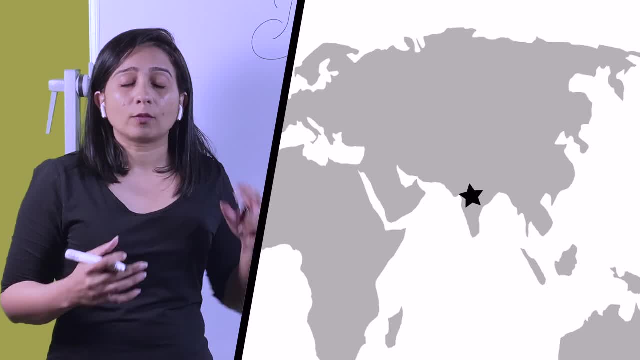 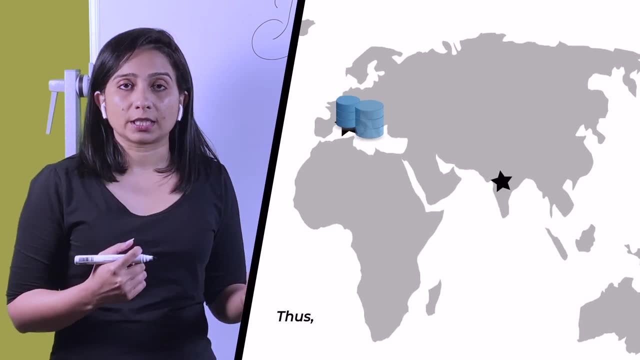 how network latency plays out. If someone is sitting in India and wants to access a file or data which is stored somewhere in Ireland, it is going to take a lot of time And in such cases replicas help If that data is replicated and kept over different geographical locations. 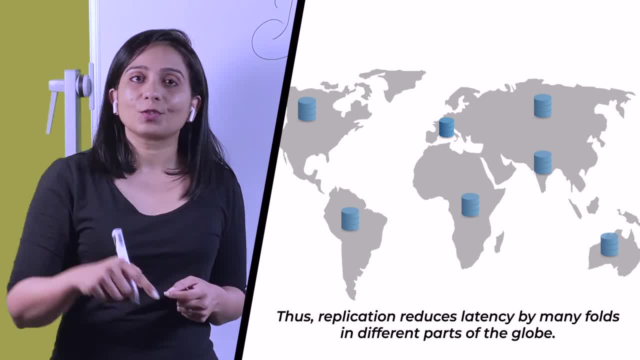 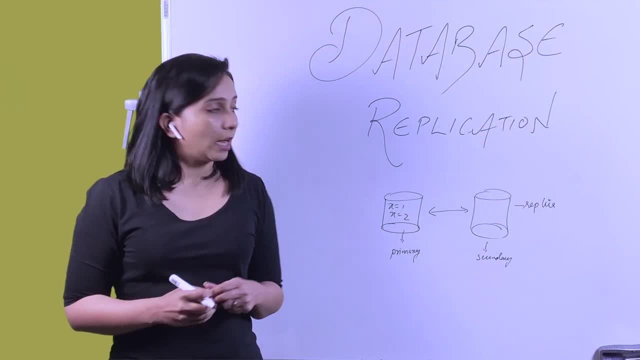 accessing that data becomes easier and thereby it reduces latency a lot. So that is the second use case, or the second advantage of having a replica. Another one is: if you have replica, it is very easy and very you know common practice to follow. 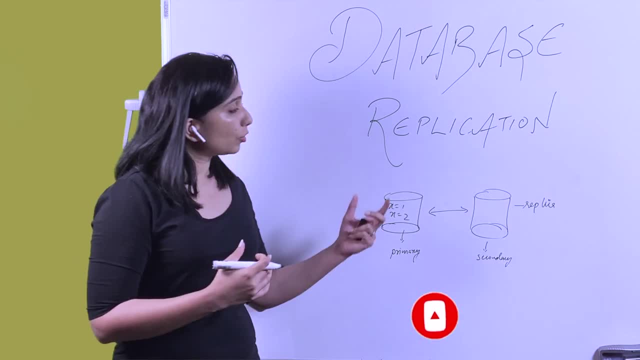 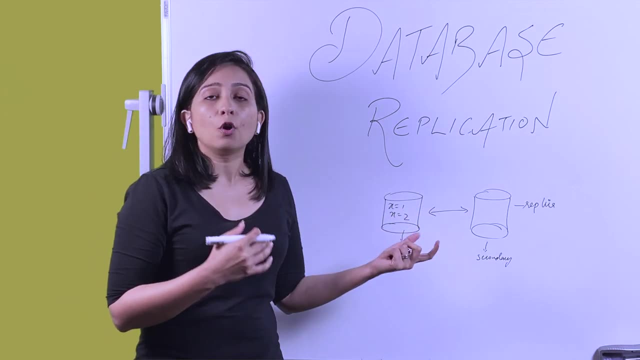 that your primary database handles all the writes and updates and your replica DBs can be used as read replicas. When I say read replica, I mean that the other DBs can be used for directing read queries, For example. let's take a real life example. 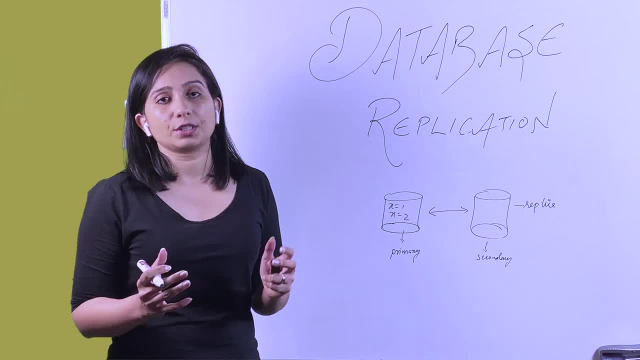 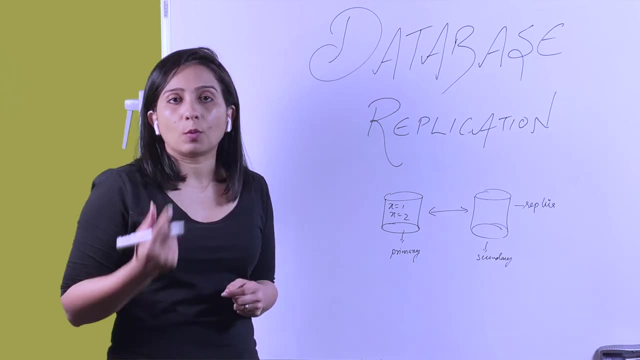 There is an e-commerce system and there is a DB which saves all the orders coming into that e-commerce system. Now the entity or the service which is updating the order might be only one: The website page or the e-commerce site page. 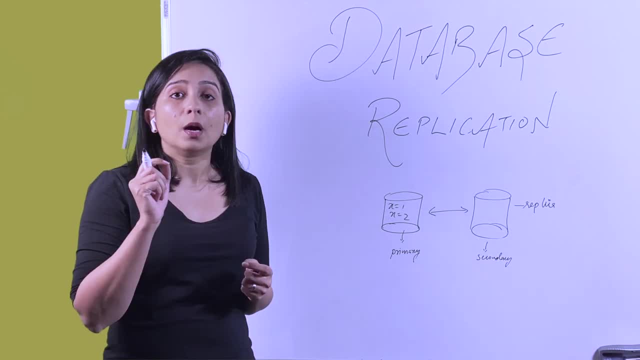 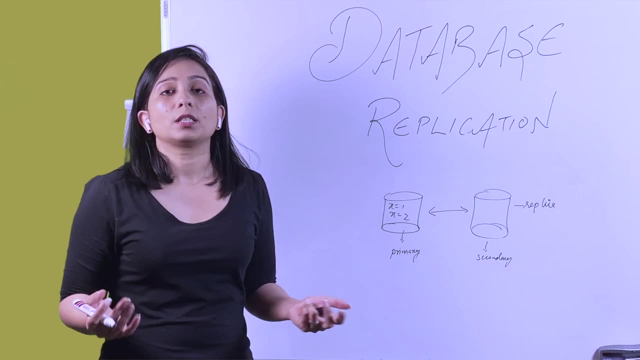 which handles the updating of the order and placing of the order. But- and it can also- there can be some other entities also which are updating the order, But there will be multiple entities or multiple services in the ecosystem which have to read the order. 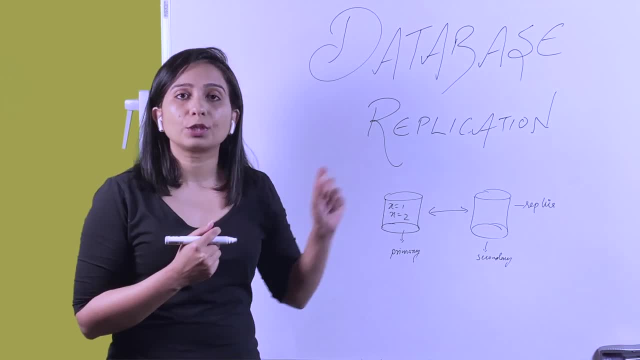 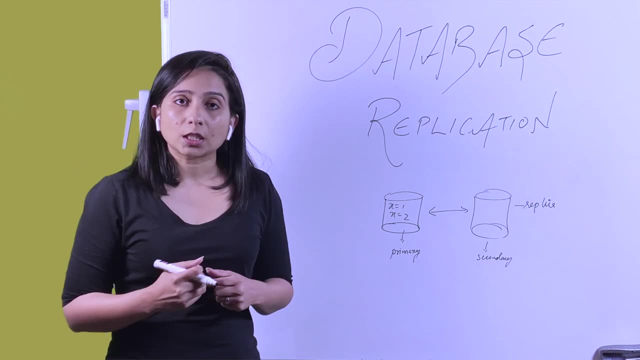 You know, let's say there is a service which generates invoice. that has to read from the order database. There is a data team which has to run analytics. They also have to read from order database. There is a marketing team which has to. 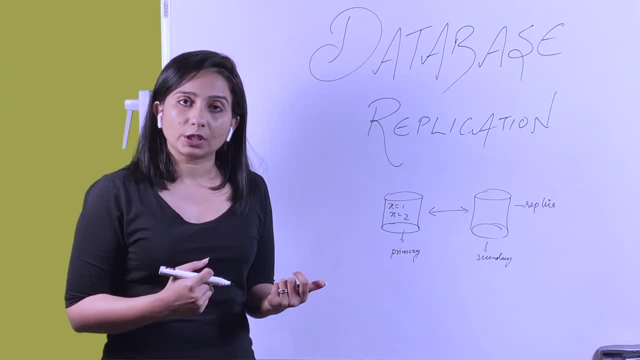 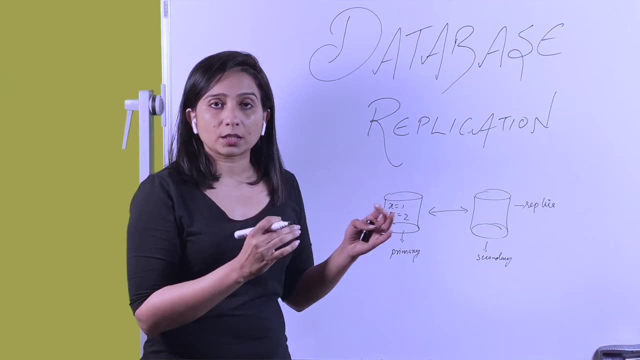 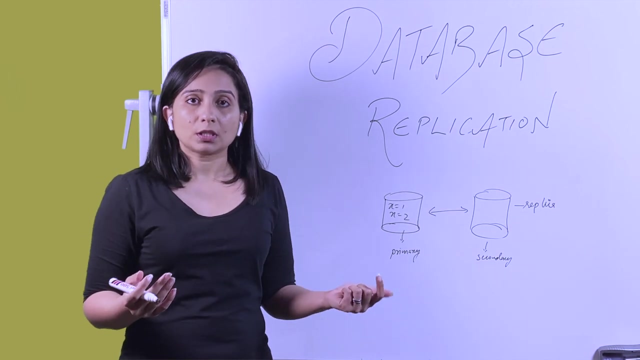 you know, run some marketing campaign depending on the orders They also have to read from order database. What can be done? Having multiple DB replicas, you can enable such other entities or services in the system to perform dates. So having replicas also allow you to increase application performance. 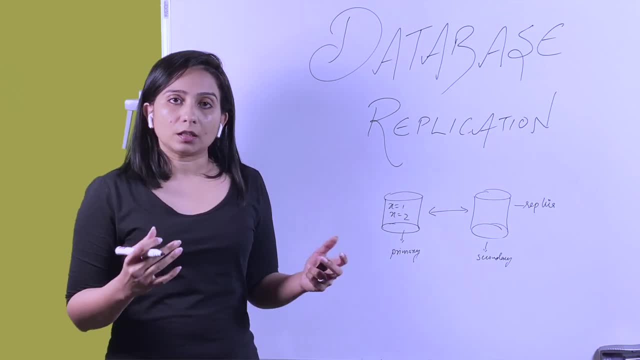 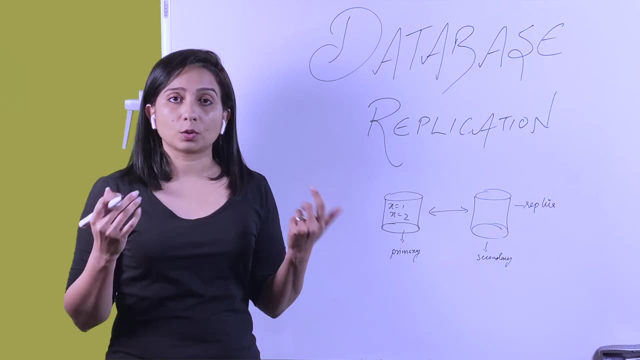 and increase the system scalability. So these three are the basics, or the basic use cases or advantages of having replicas. So far it all sounds good and it all sounds very advantageous, But there is a lot of complexity that comes while handling the replicas. 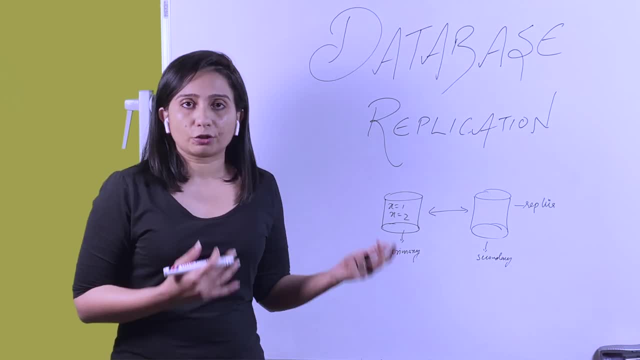 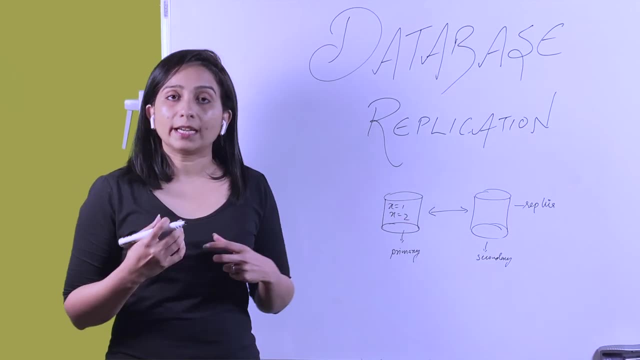 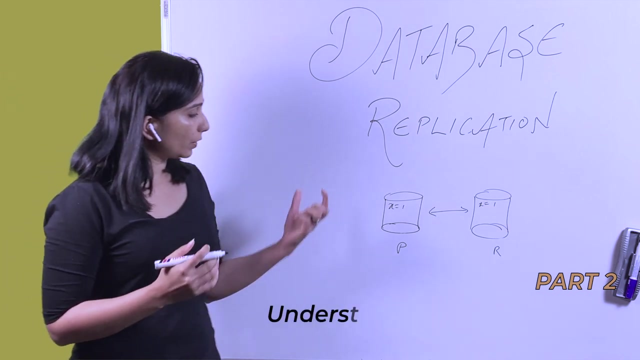 and updating the data and making data available across all replicas. Let's see why that happens. Let's take a simple example where we have one primary database and one replica. Now let's say an update comes at time, which means that we have one primary database and one replica. 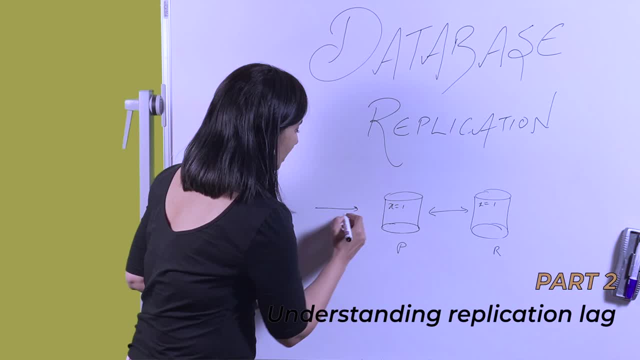 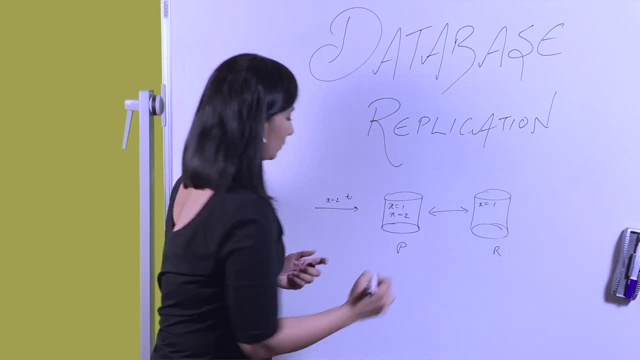 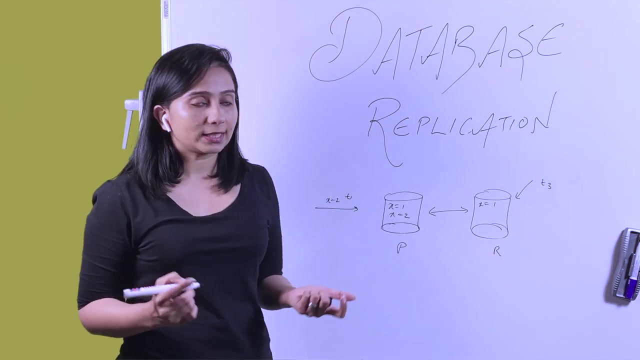 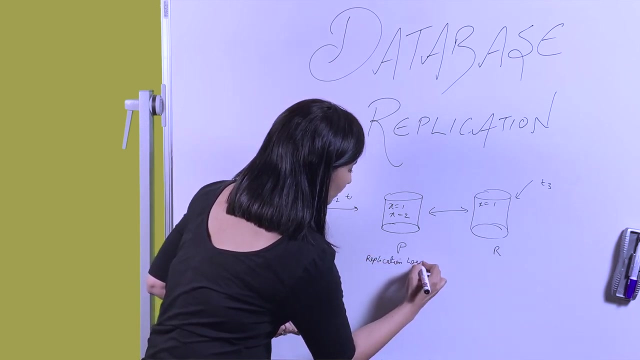 Now let's say an update comes at time, at time t1 to primary- and this value is updated And at the same time a read request comes here at t3. Now let's see what happens. Let's say the value of replication lag is R. 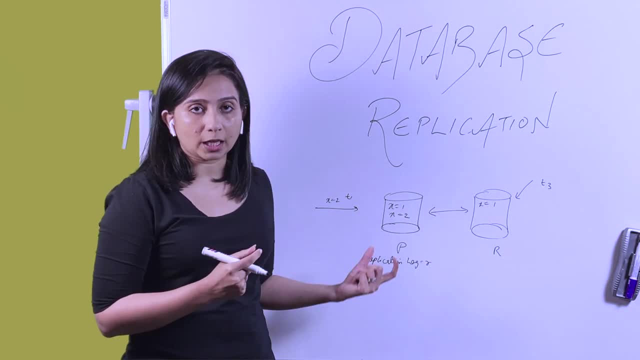 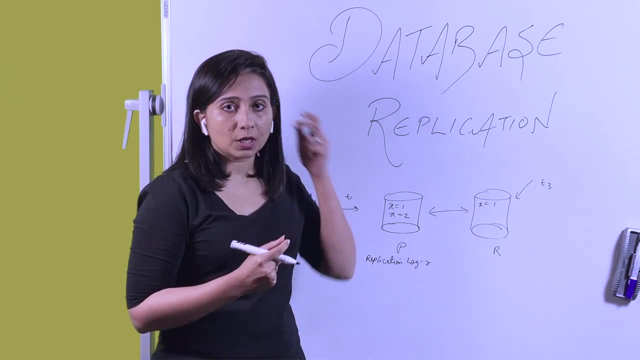 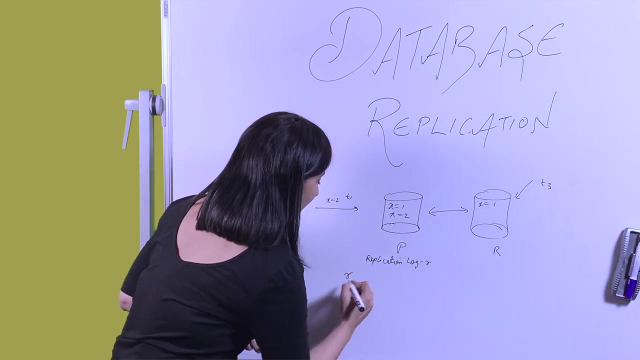 Now, what is replication lag? Replication lag is the time it takes for the value to be copied from primary to secondary database, Or the replica. So let's say the write happened at t1 and the read happened at t3.. If replication lag is less than t3 minus t1,, 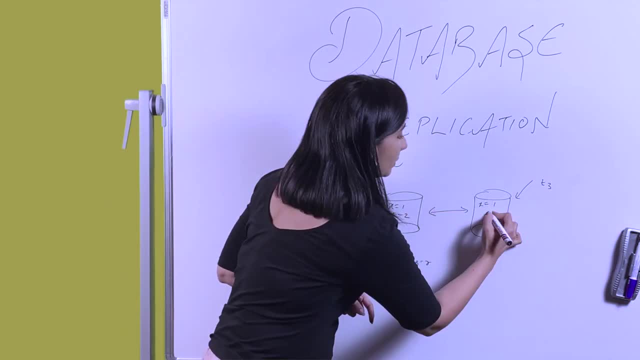 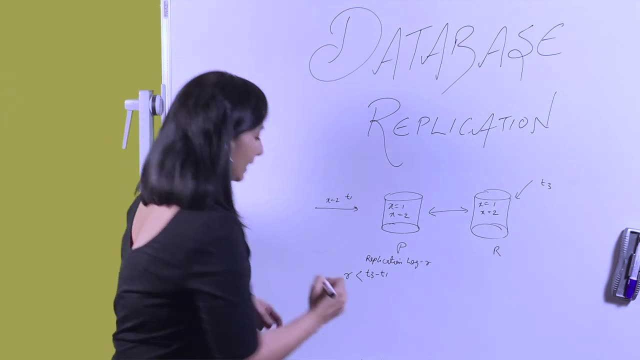 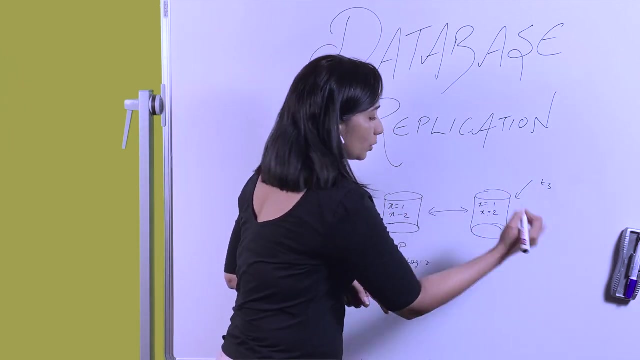 that means at time t3,, the value of x will be updated And when the read happens the user will get to see the correct value. But in case replication lag is greater than t3 minus t1,, then at t3, still, the user will be able to access the value x equal to 1.. This is okay if replication lag is lower. Let's say replication lag is in the order of, say, milliseconds, The system can still access the value, but with a lag of, say, 1 millisecond or 2 milliseconds or 10 milliseconds. But if the replication lag is huge then it becomes a problem. 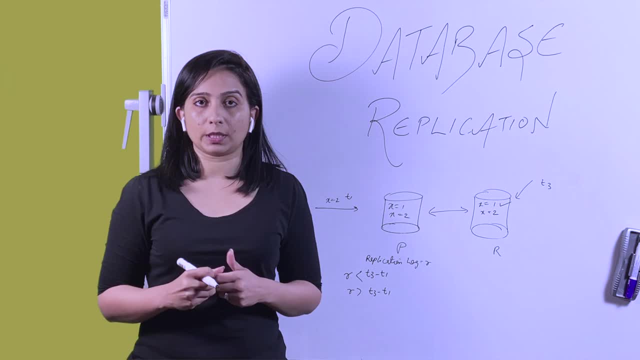 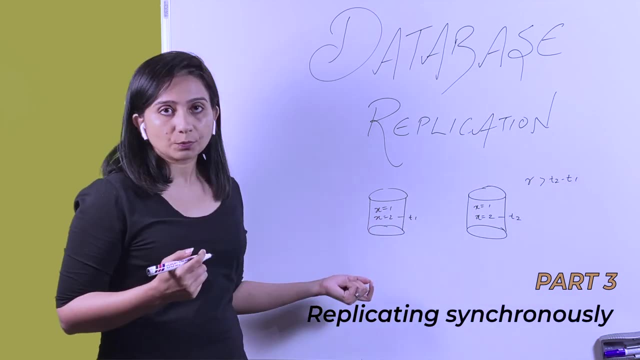 And this problem becomes worse when there are n number of replicas. So how do we solve it? Let's see So, as we just discussed, that a write was issued at t1 and the value was sent to replica was written, updated in replica at t2.. 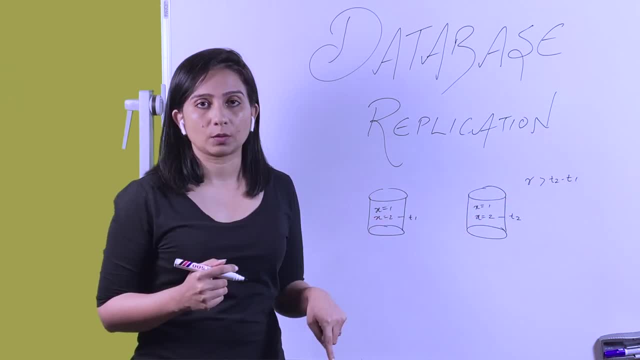 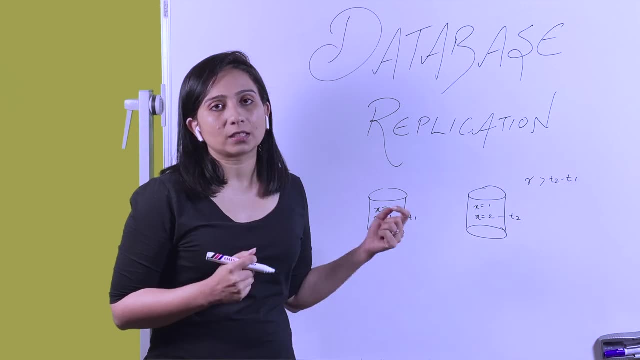 And let's say the replication lag is higher than t2 minus t1.. In that case what would happen? The entities of the services which are reading from this DB will end up getting inconsistent data. If someone is reading from master itself, they will get x equal to 2. 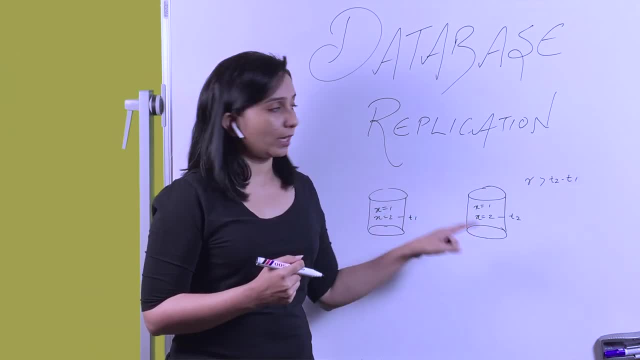 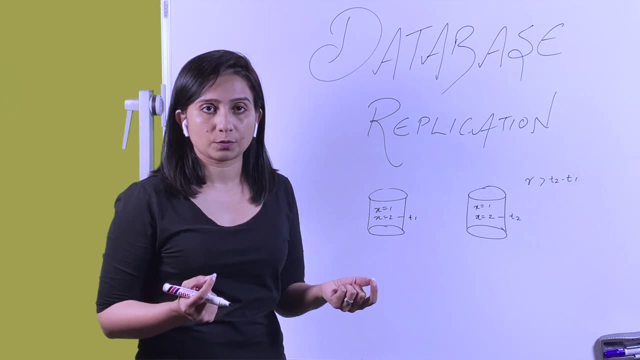 and if they are reading at t2 from replica, they will get x equal to 1.. So this is the state of inconsistent data: For the same value of x, people are getting two different values. Now the challenge is to solve this consistency issue. 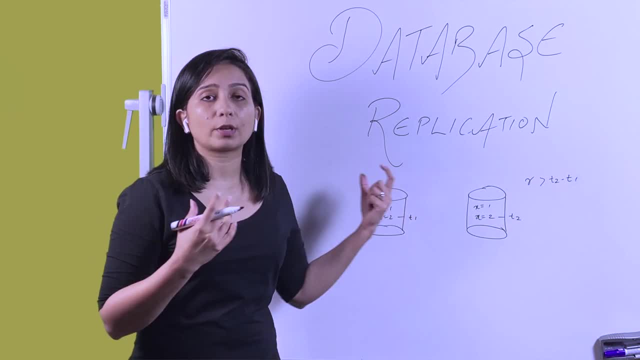 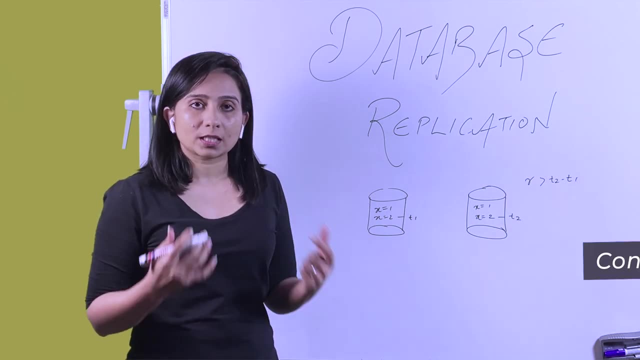 and design the system or build the reads and writes or replicas in a way so that the data is consistent at all times. The way these problems are solved are known as consistency models or consistency algorithms. I will just give you a brief idea about one of the consistency models. 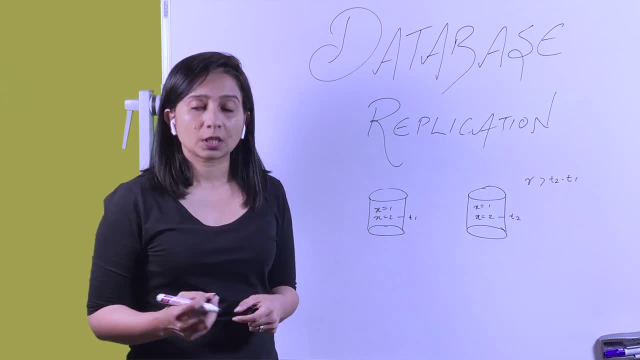 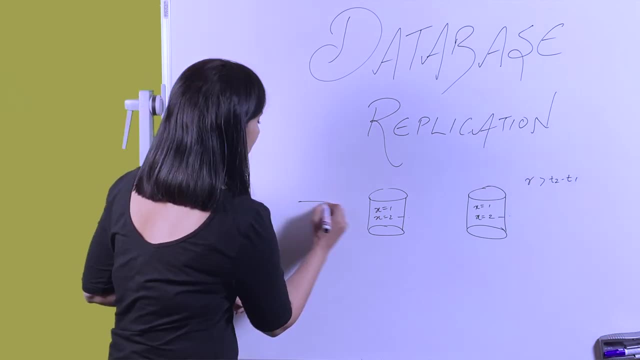 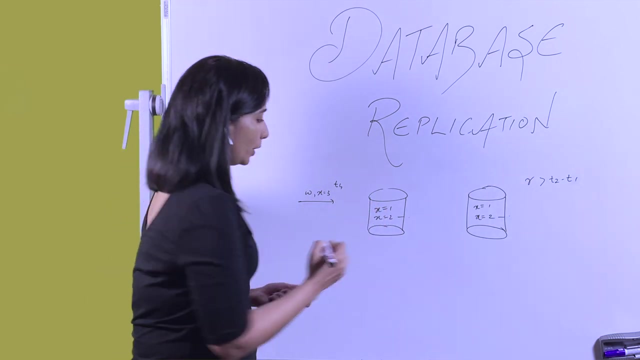 It is called read after write consistency. Let's see what that is. Let's say, forget about t1 and t2.. Let's say a new write is issued, x equal to 3 at t4.. Now what primary DB is going to do? 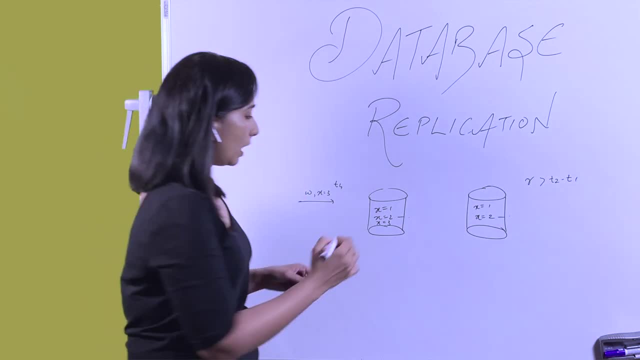 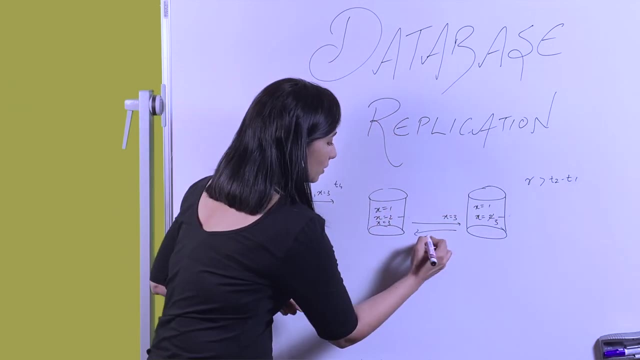 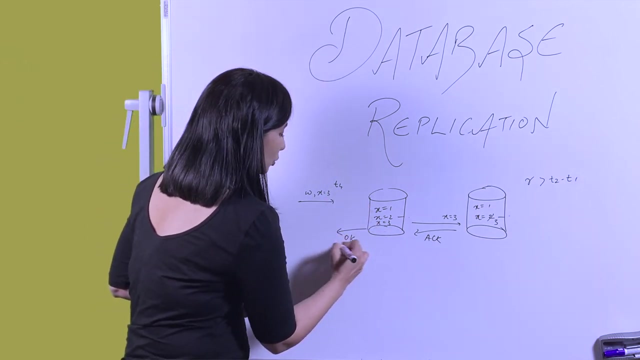 It will update x equal to 3.. Then it will ask replica also to update x equal to 3.. Then replica updates the value and acknowledges the primary that I have updated the value And once that happens, the primary says to the issuer of the write. 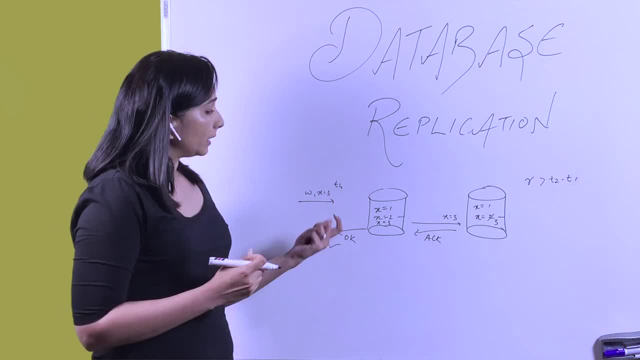 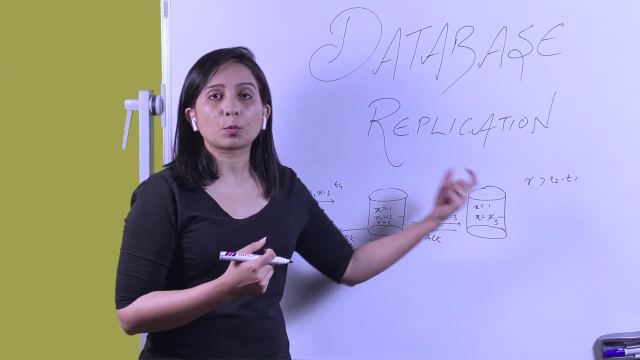 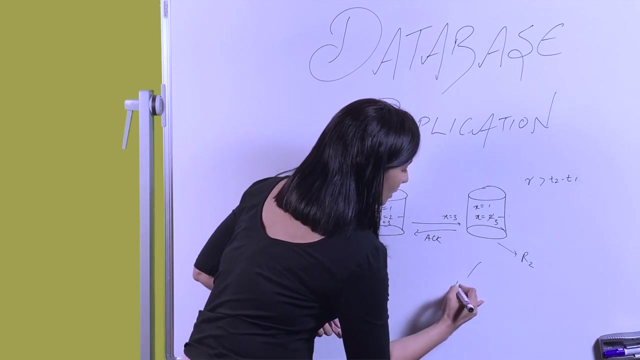 that your write has been completed. This means that the system or the user will not see write is completed until unless the write value has been propagated to replica as well, In this case if there are multiple replicas, say R2, R3 and R4,. if this strategy of read after write is followed, then while sending updates to replica, master will send updates to all the replicas, wait for all of their acknowledgment and then it will tell the write issuer that write has been completed. In this case, replication lag is zero. 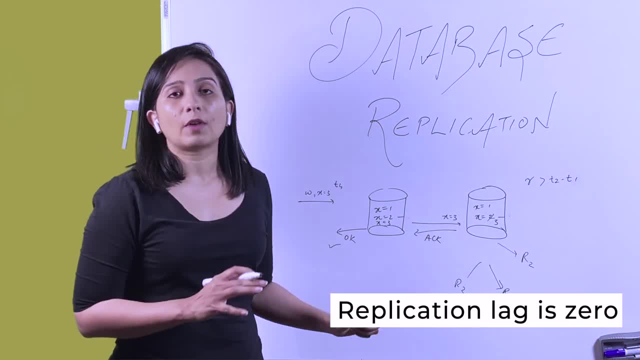 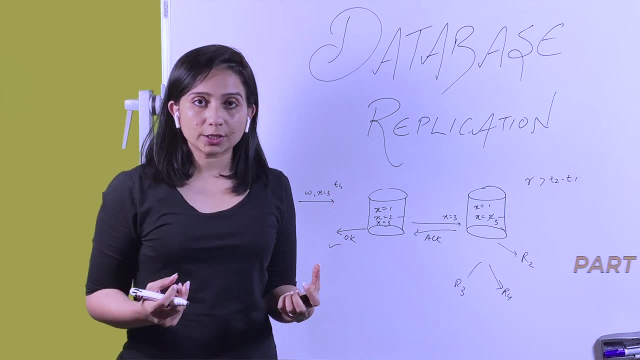 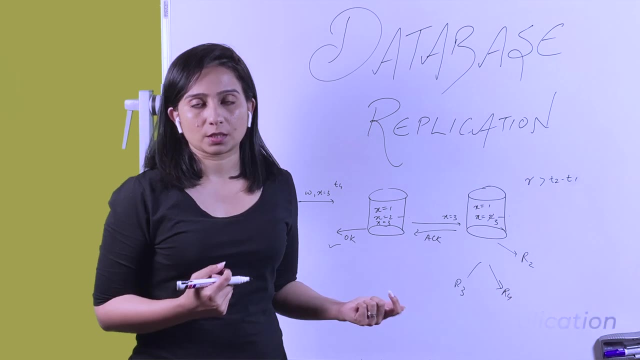 Why? Because the master is taking care of updating the values to all the replicas and not declaring the write as complete. This is also known as synchronous replication. The advantage of synchronous replication is that, first, the lag is zero and, second, the data is always consistent in the system. But what is the downside? The downside is that the performance might take a hit because every write will have to wait for all the replicas to get updated and as well as acknowledge to the write issuer that the write has been done. So it will take a slightly higher time. 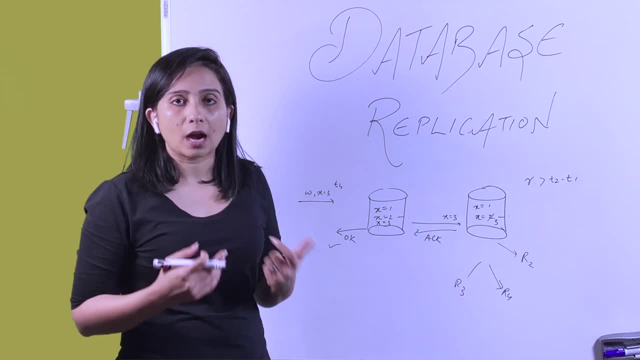 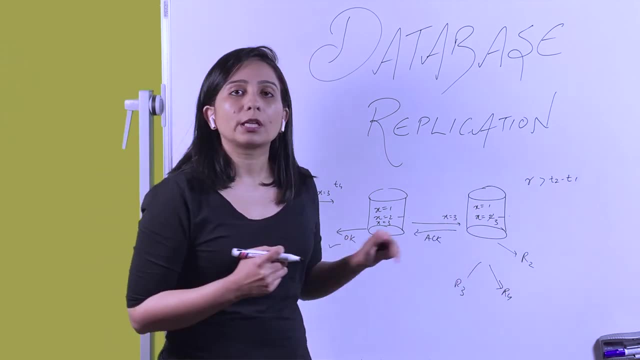 or I would say that the latency of that whole write operation is going to be higher because it's waiting on the other replicas And in case of failure scenarios any of the replica goes down and fails to acknowledge. Let's say: master said new value of x is 3,. 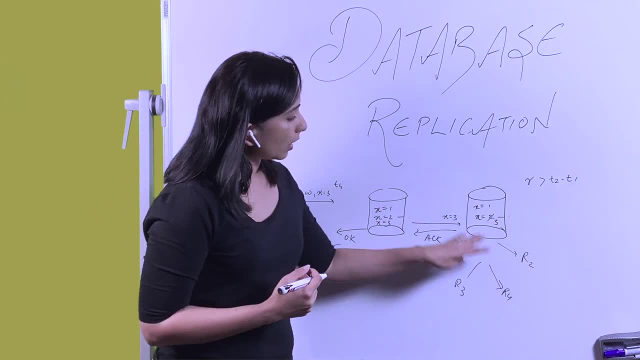 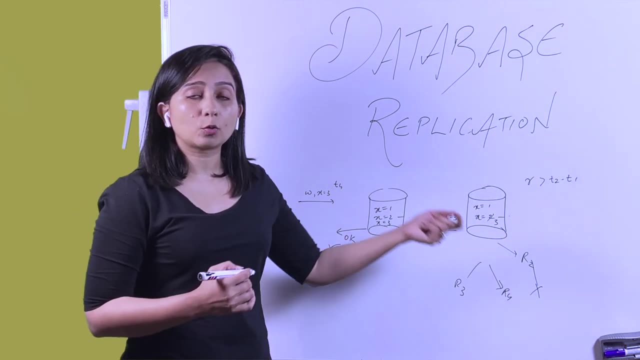 so replica 1,, 2,, 3,, 4,. please update x equal to 3.. So R1, R4 and R3 updated, but at that same moment R2 failed and R2 couldn't give an acknowledgement to the master that I have updated the value. 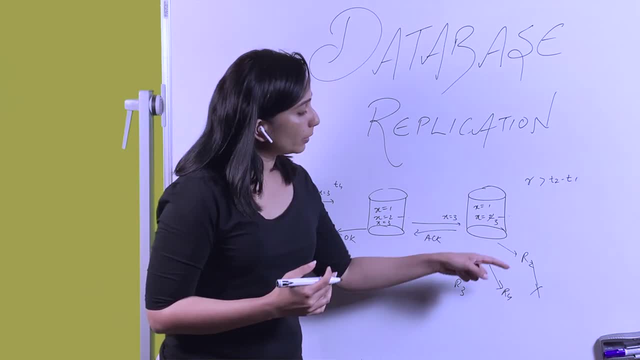 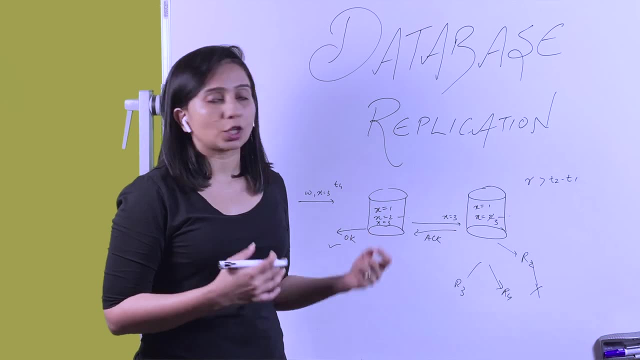 and in that case write will fail. Now you would think that the probability of this happening is not that high, but we should not think in those terms that what are the chances of happening this? Either we should think in terms: what would be the consequences? 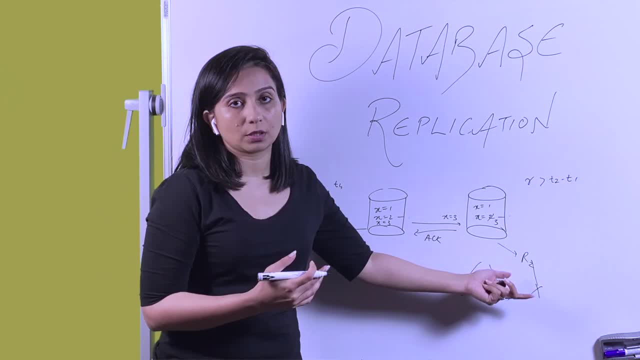 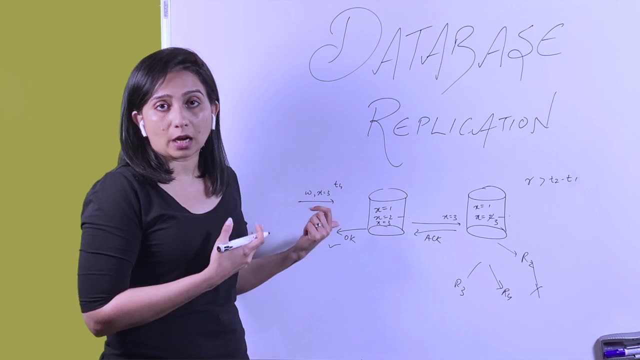 or what would be the challenges we will face if this happens, If one of the replica misses write and if one of the replica goes down and the writes are not happening or the writes are blocked because one of the replica went down. So this is the failure scenario that we have to take into consideration. 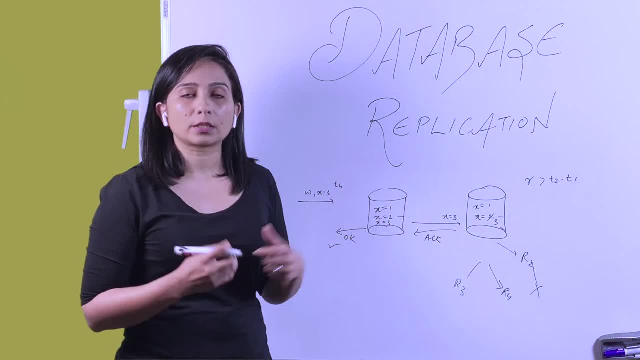 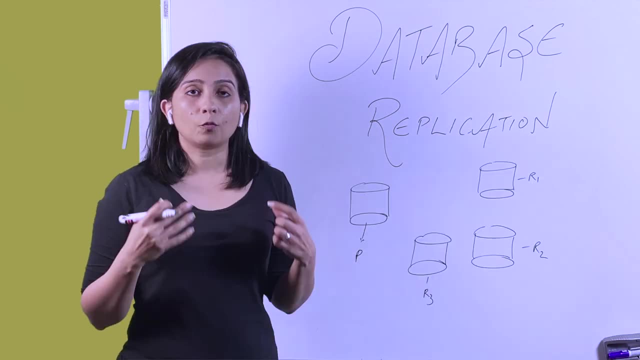 and this is the disadvantage if we go along with synchronous replication technique. Now, how can we solve it? Is there an alternate to synchronous replication? Yes, let's see what it is. One more way of replication other than synchronous replication is asynchronous replication. 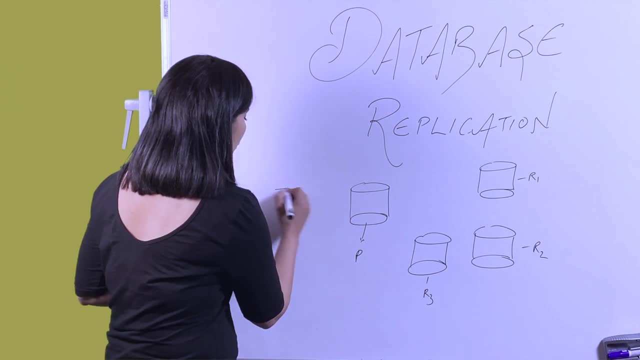 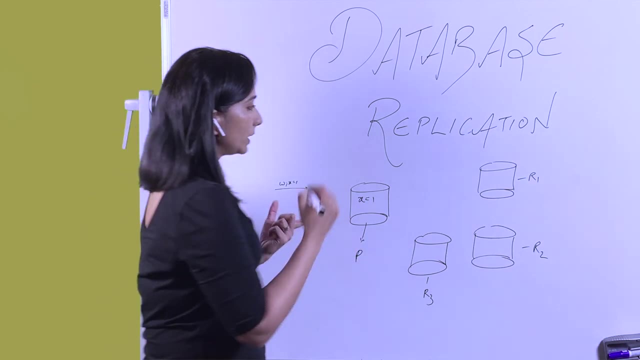 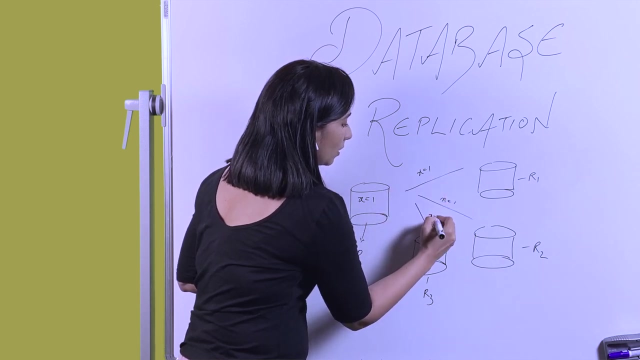 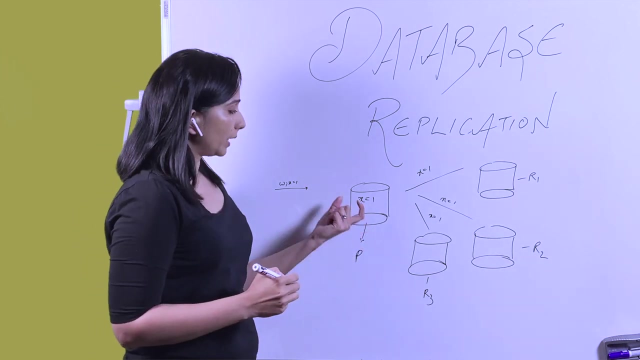 Let's see what would happen in asynchronous replication. A new write is issued. In this case the primary will send a message to all the replicas to update x to 1. But it wouldn't wait for the acknowledgement from any of the replicas, and just after the value is updated in the primary DB. 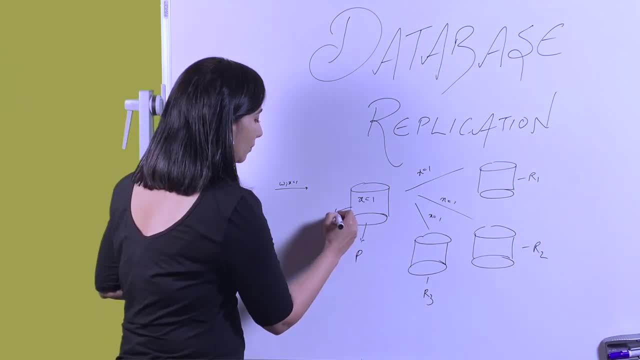 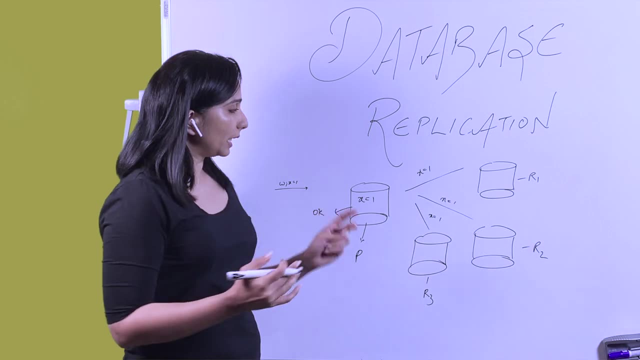 and a message is sent to the replicas, it will say that write has been completed. So this is called asynchronous replication. The replication is still happening, but it is happening in the background. The primary DB is not waiting for the acknowledgement of replicas. 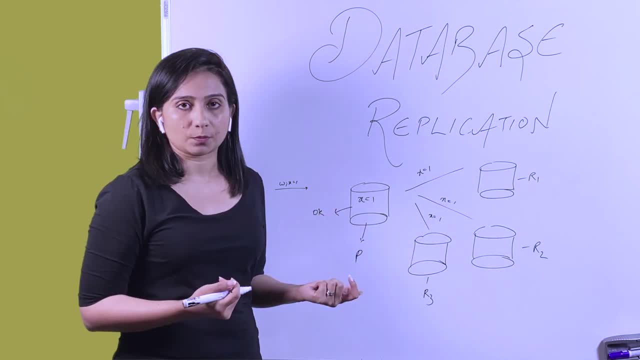 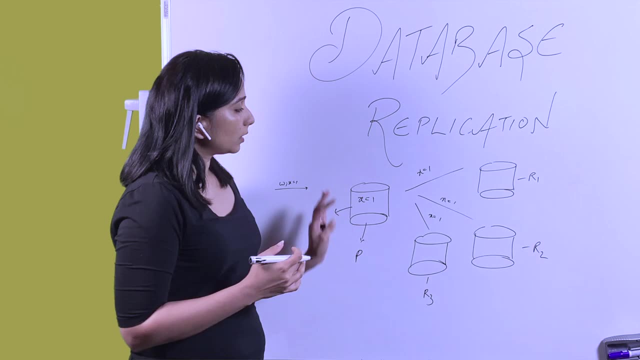 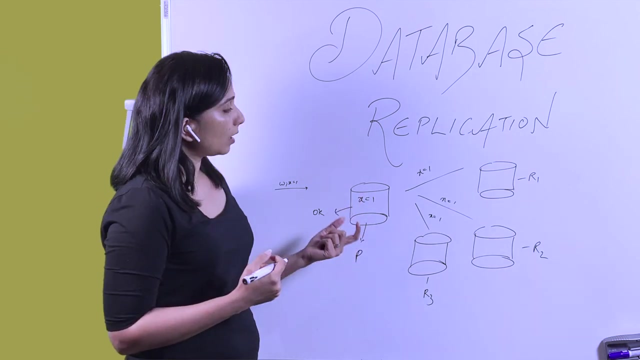 The advantage: the write operation becomes faster. The disadvantage is that if any of the replica fails or it doesn't update to the value, the system will end up in an inconsistent state. But if there are a number of replicas, then again we can ensure that at least some replicas will have correct values. 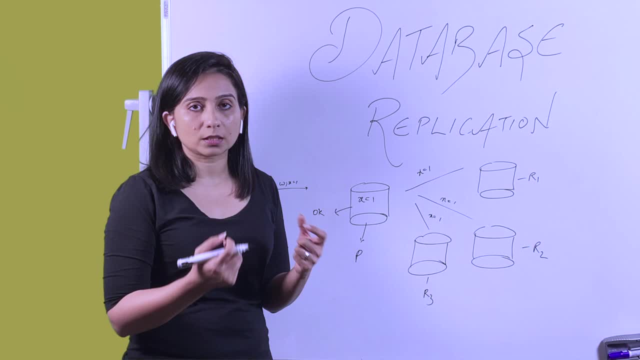 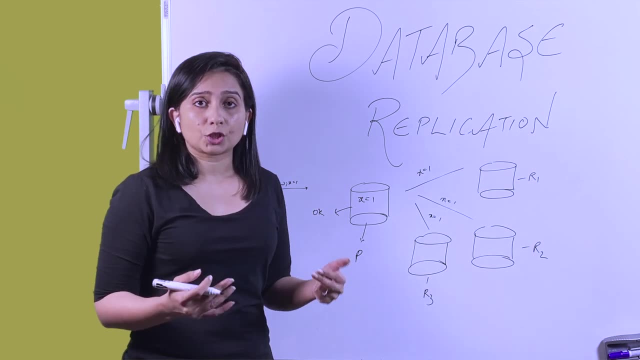 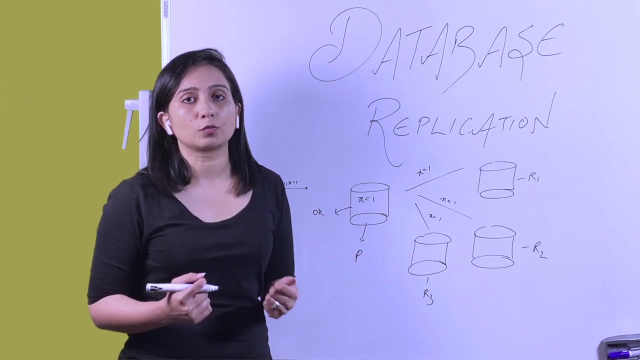 and we would have to face the inconsistency of data in some cases or in some replicas. Again, it depends on the business use cases. If it's a banking application or if it's a flight application, where the consistency is of highest importance, this model might not be useful. 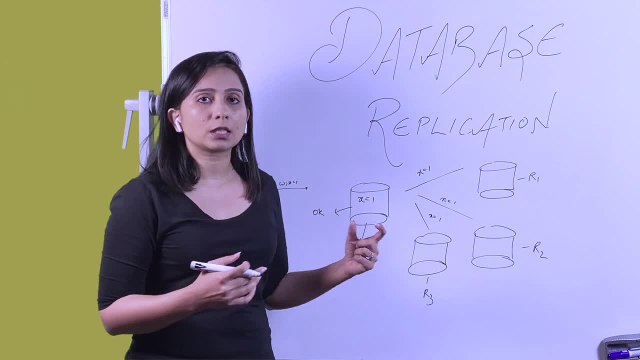 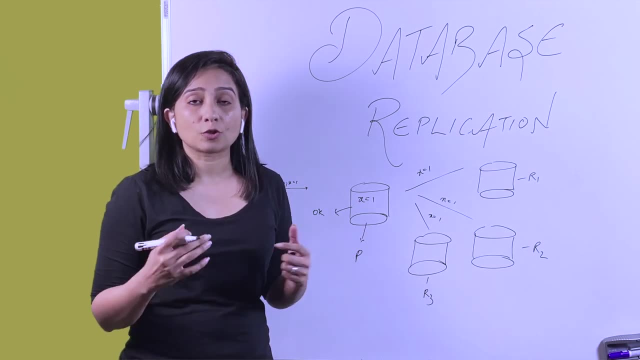 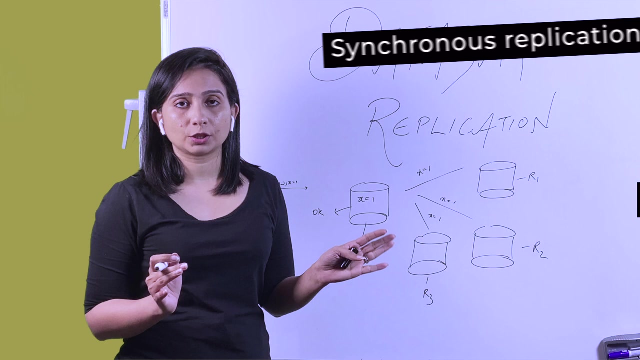 But if it is a business application where the data consistency, with some inconsistencies, are okay, or the updating of the data can take some time and accessing real-time data is not of utmost importance, then this approach can be followed. So we discussed two approaches: Synchronous replication, where we are waiting for all the replicas to acknowledge. 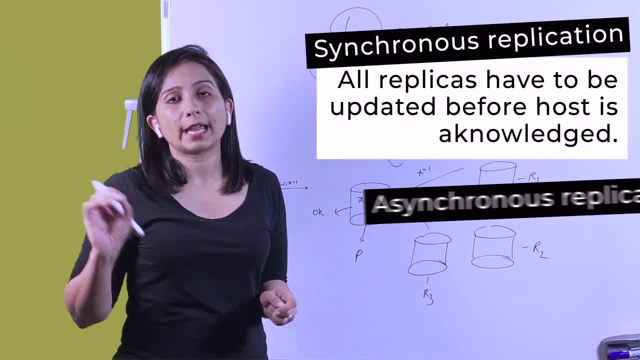 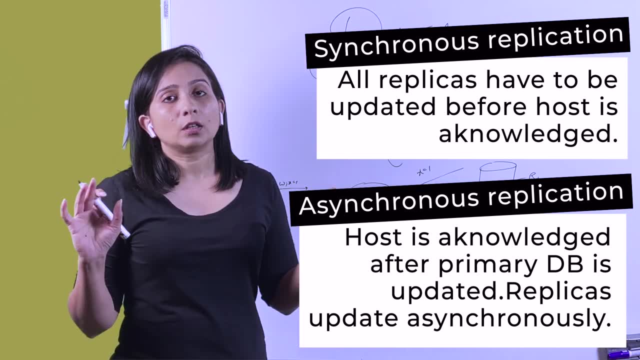 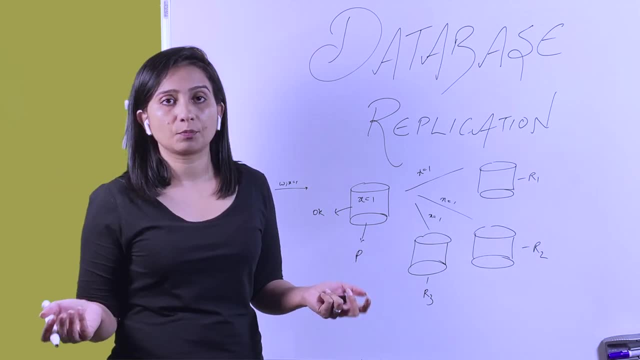 and asynchronous replication, where we are not waiting for any of the replicas to acknowledge, We are just depending on the primary DB to update the value and return. Now, both these approaches have their own pros and cons, like as we just discussed: One gives performance, one gives higher consistency. 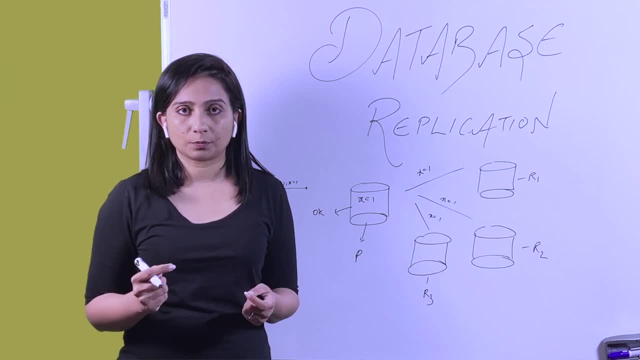 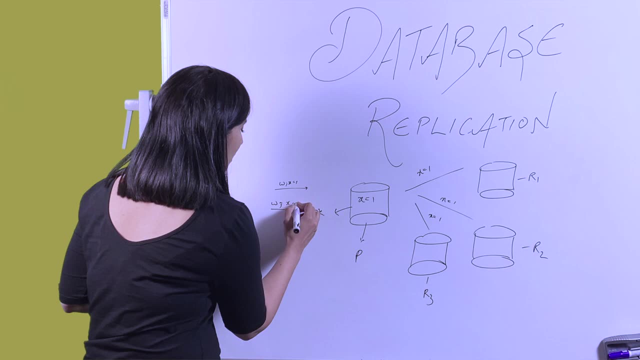 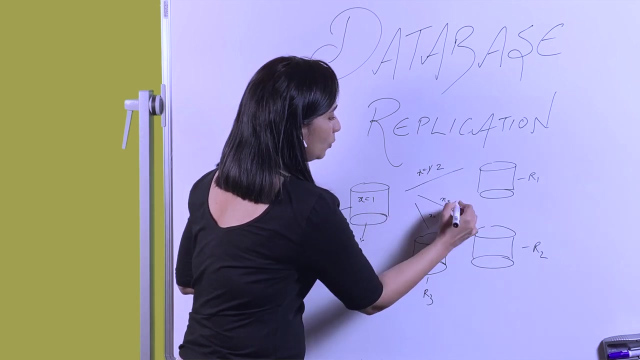 Now there is a hybrid approach, which is also called as semi-synchronous replication. In that case, what happens is, as soon as a new write is issued, say x equal to 2, the primary DB will update the new value to all the replicas. 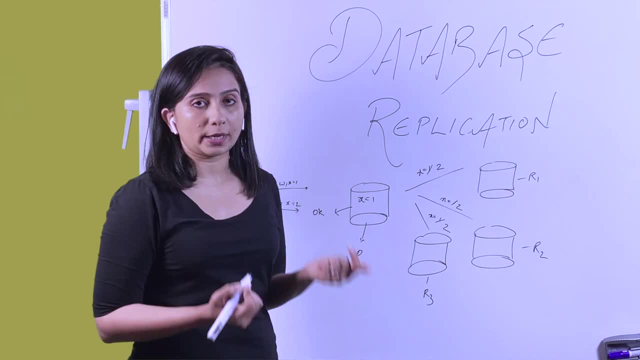 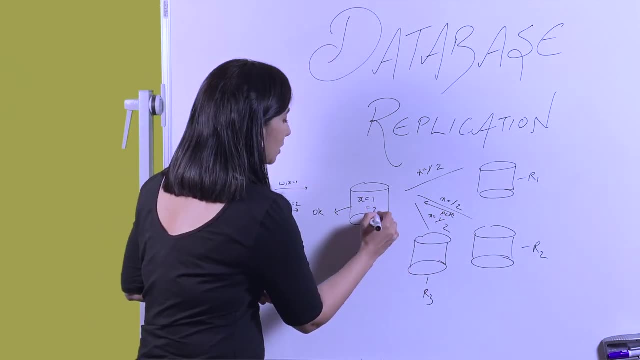 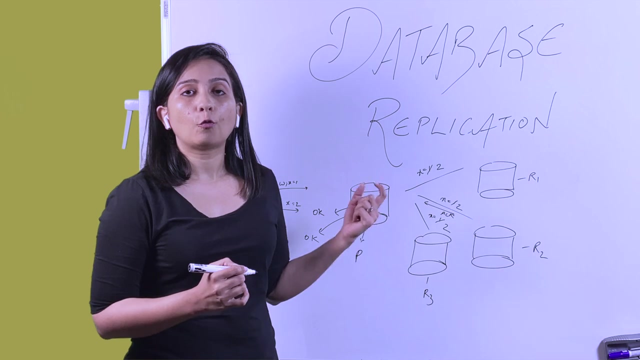 and will wait for only one of the replicas to acknowledge. Let's say, R2 acknowledges that x equal to 2 has been updated. In that case primary DB also updates and says the write has happened. So here the primary DB is waiting for one replica to acknowledge. 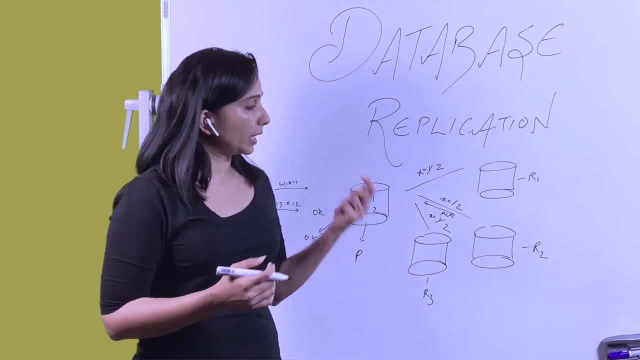 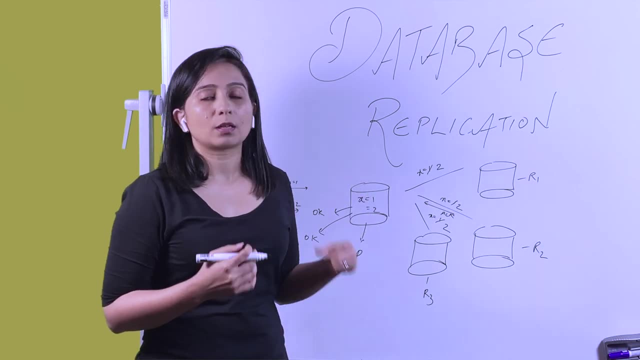 In some cases, when these systems are implemented, in some cases the primary DB waits for one replica, and in some cases it can be 2 or 3 or n. This number is also known as quorum. Again, I am not going into the in-depth of replication. 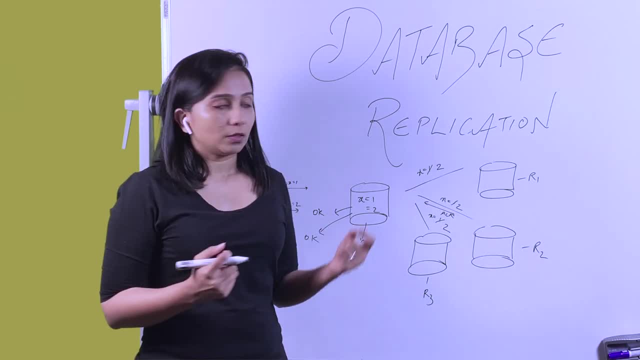 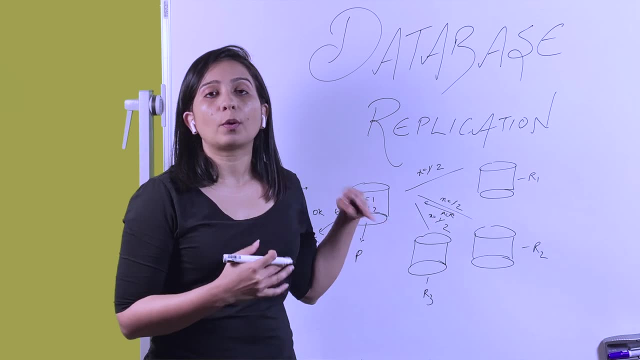 but I am giving you an idea to build upon. So here we are, waiting only for one of the replicas to acknowledge, and then we are relying on other replicas to update in background Here. if any of the replica fails, we are okay because it is updating in the background. 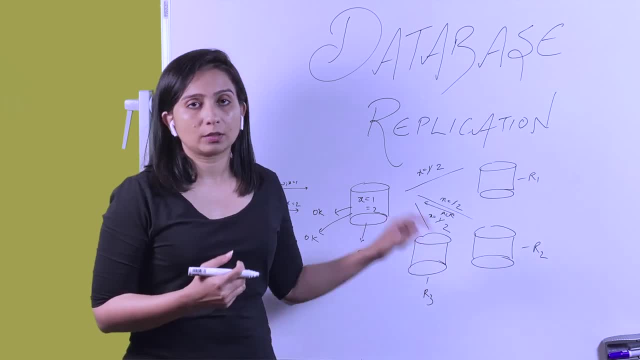 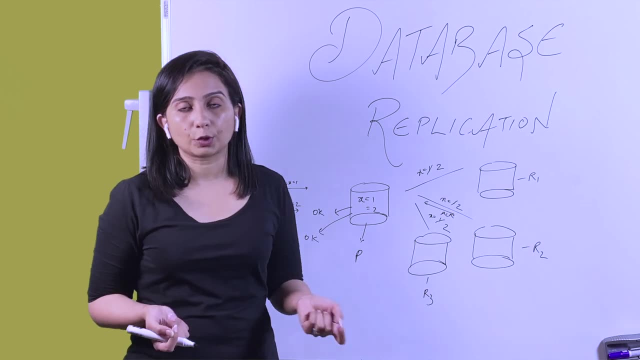 If the replica that has to acknowledge if that one itself fails, then again we are in a problem. But also we are able to serve writes faster here because we are waiting only for one of the replicas. So since this is a hybrid approach, 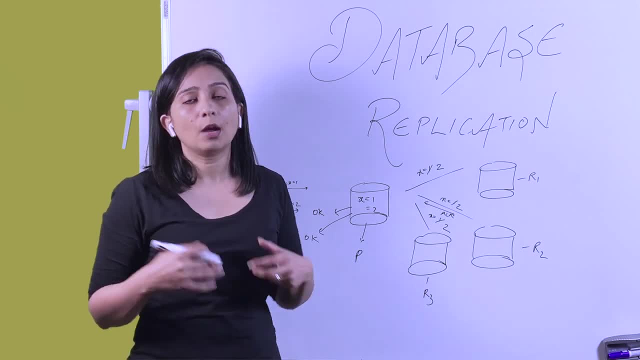 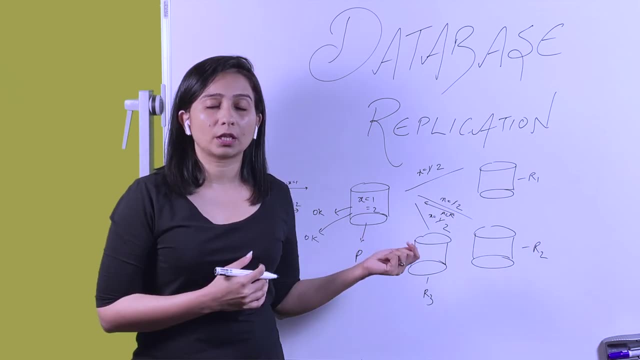 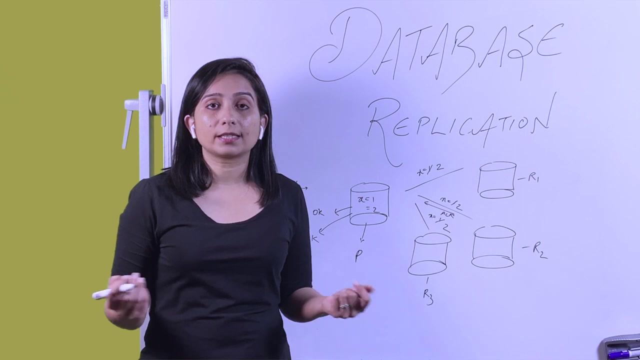 it has some positives of synchronous and some positives of asynchronous, But again, it has its own caveats. Now the question arises: what kind of consistency model or what kind of replication approach is chosen when DBs have to be replicated and when large-scale systems are designed? 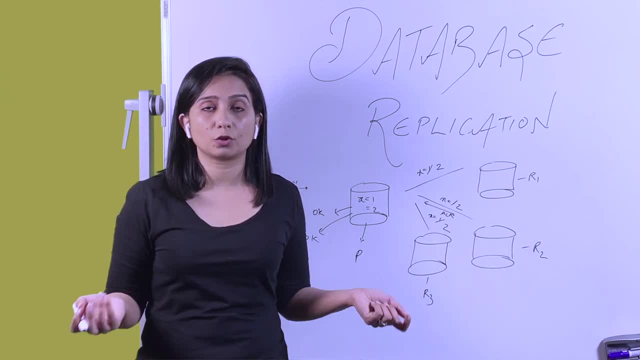 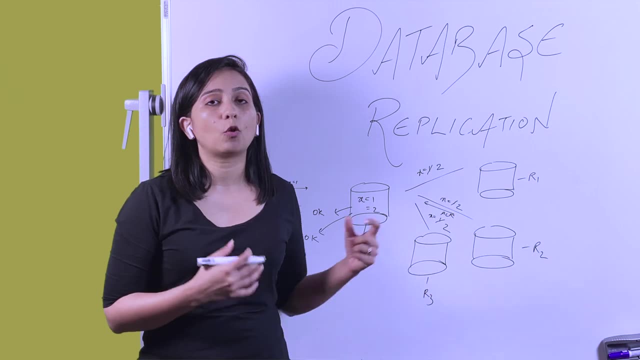 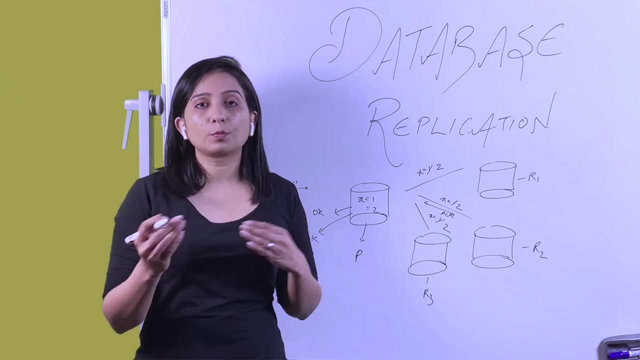 where the DBs are distributed across different geographical areas. Good news is there are a lot of scalable systems which exist which implement one of these or a combination of these algorithms to maintain a high consistency model and high availability. But again, you have to choose between one of the trade-offs. 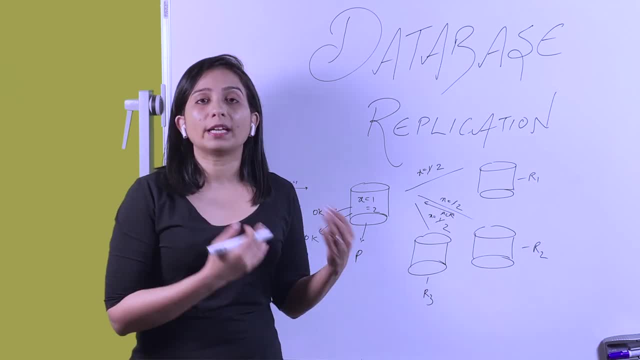 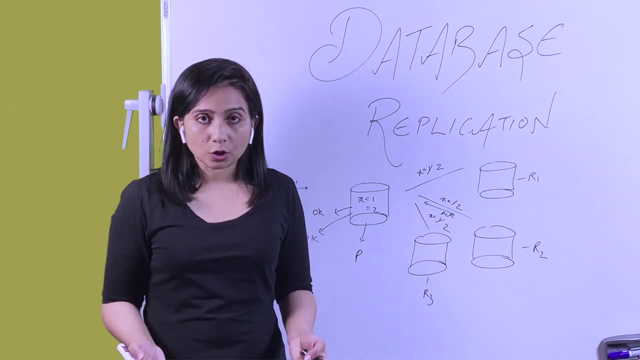 Either, if the performance is of highest importance, you might have to give up on consistency. If consistency is of highest importance, you might have to compromise on performance or you might have to incur extra cost. It depends on the use cases. I would like to tell you that this replication and consistency 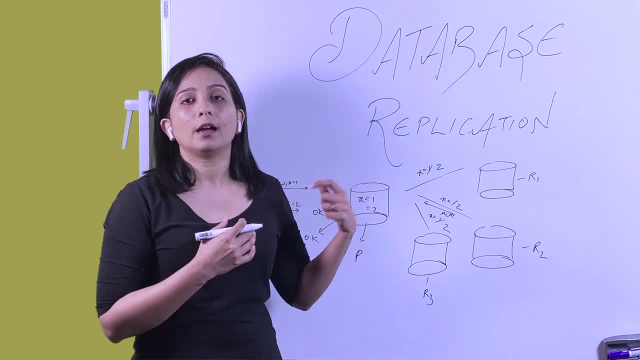 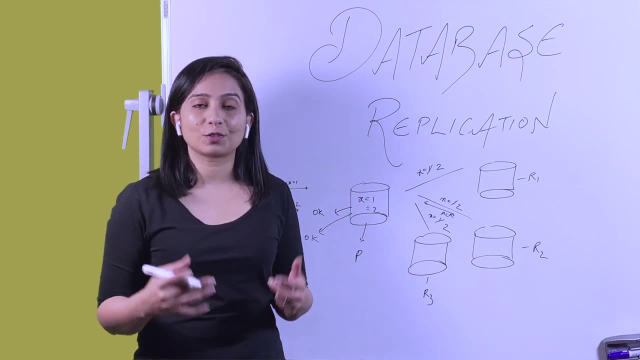 and how replication is helping in fault tolerance and reducing network latency and increasing the performance. some of these concepts also form the basis for one of the next videos, which is the famous CAP theorem. So I would like you to absorb these concepts And, if you have any slight doubt in any of the part, 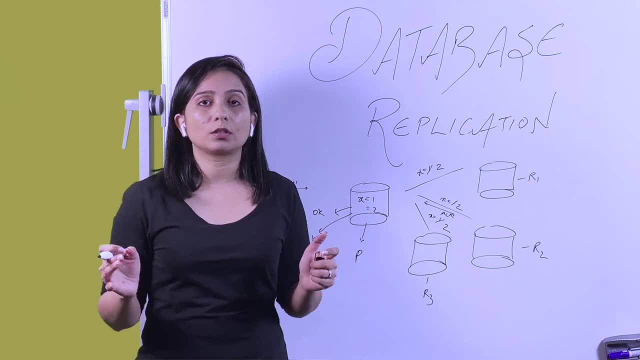 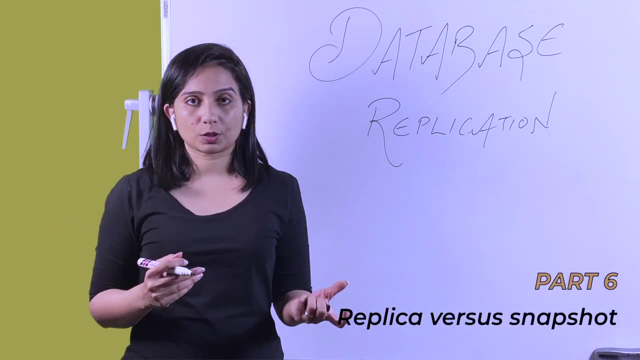 please feel free to comment and ask me so that we don't end up having wrong information, Since we are talking about replicas. one of you will have a question about snapshots And you might think that is a snapshot same as a replica, or what is the difference? 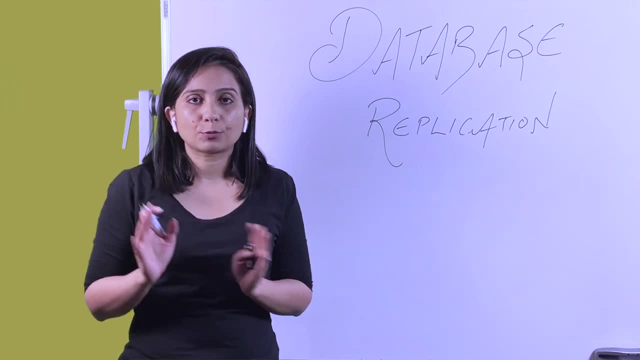 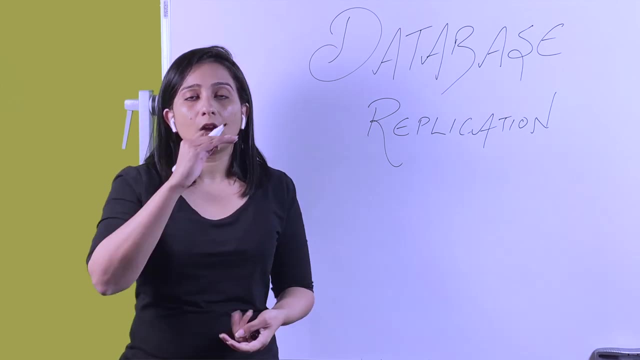 Replica can also be thought of as a snapshot, but actually a snapshot is different. You can think of snapshot as taking a state of database at a certain time, like taking a state of particular rows and the data of a DB at a particular time. 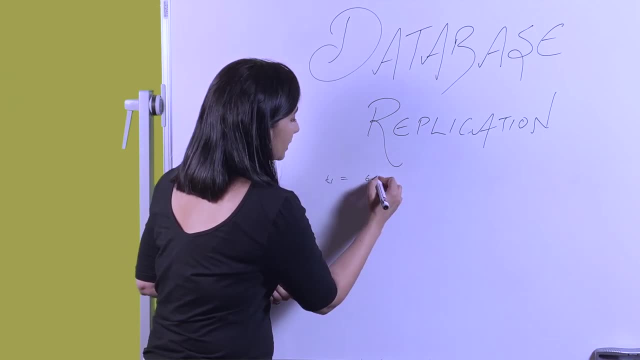 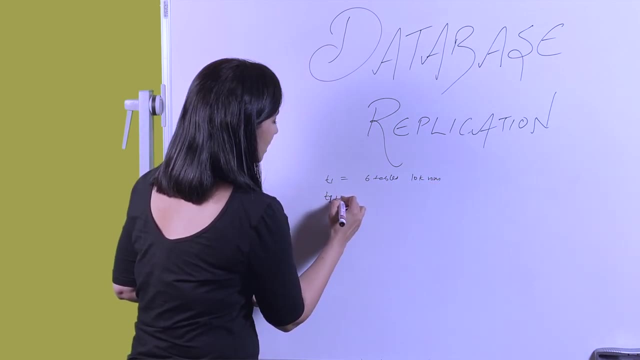 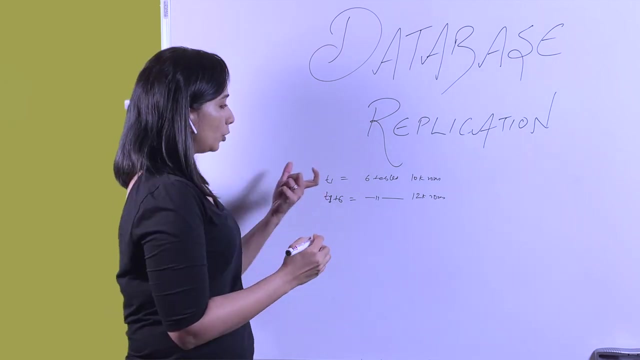 Let's say, at T1, your DB had six tables and 10k rows. At T1 plus six hours you still had six tables, but let's say 12k rows. So you take a snapshot at T1, you take a snapshot at T1 plus 6. 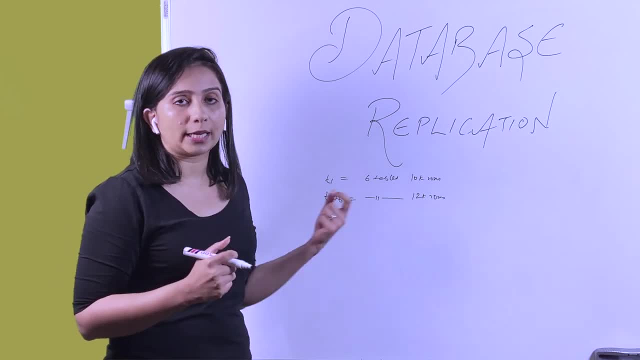 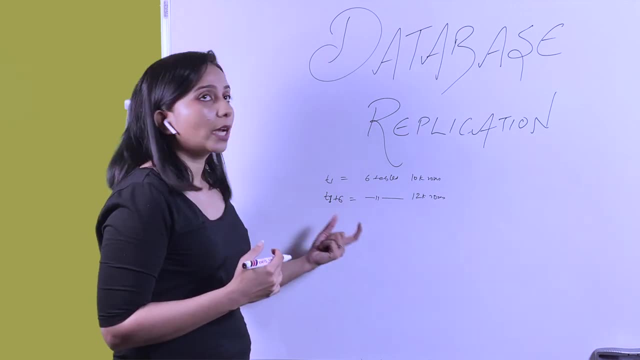 and T1 plus 12 and so on. There are different time intervals at which snapshots are taken And if something goes wrong in an unfortunate event where you lose your data, you have the snapshot of your data and you can roll back to one of these states. Having a snapshot allows you to have stored states of data so that you can recover the data in the event of a failure. Having replica, on the other hand, as we discussed, help you tolerate faults, reduce latency and increase application performance as well. 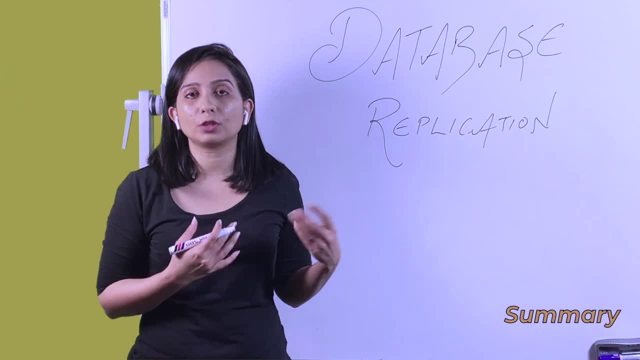 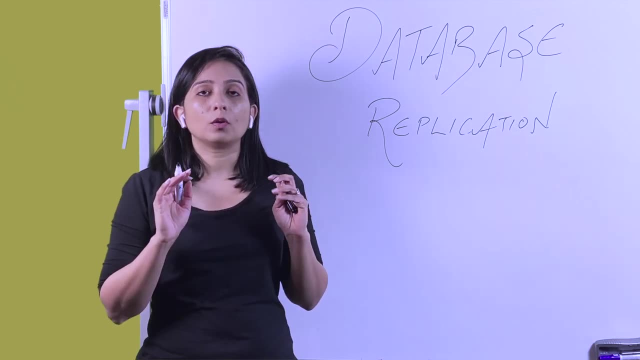 Now let me give you a brief overview of how replication is actually done. Like I said, that the master issues a message to replica, that update the value, but actually how that is done. So in reality, different systems or different databases implement replication in so many different ways. 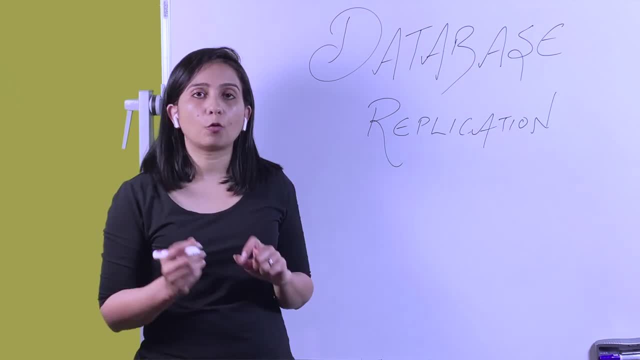 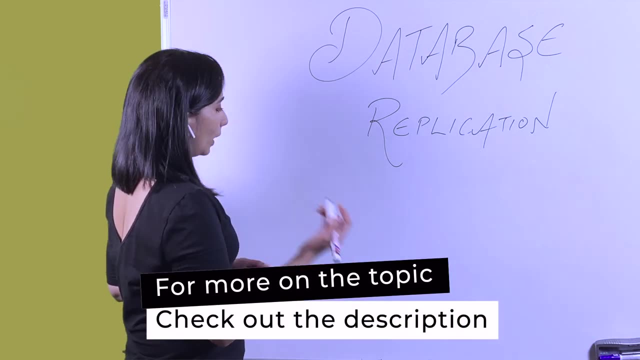 using some sophisticated algorithms, But I'm going to give you an idea of two or three ways how replication is carried out, And I have linked so many resources in the description for you to dig deep. So one way is that this is your primary DB. 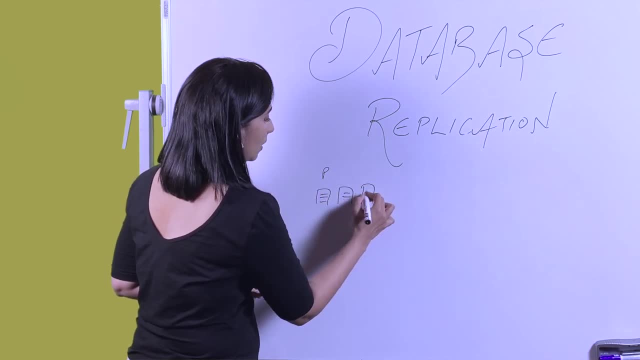 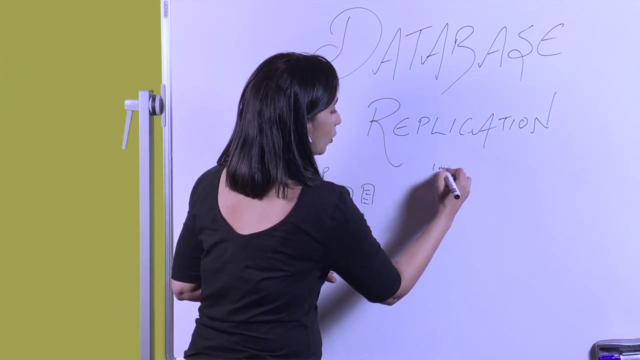 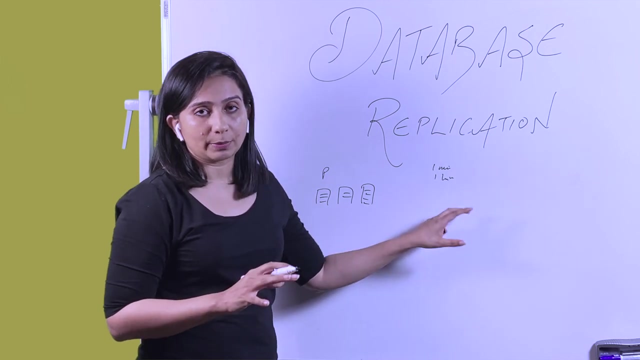 It has all sorts of tables And the replication is happening periodically, Let's say after every one minute or one hour. a job is running which is taking a capture of all these tables and dumping it into a replication DB or different copy tables. That is one of the ways. 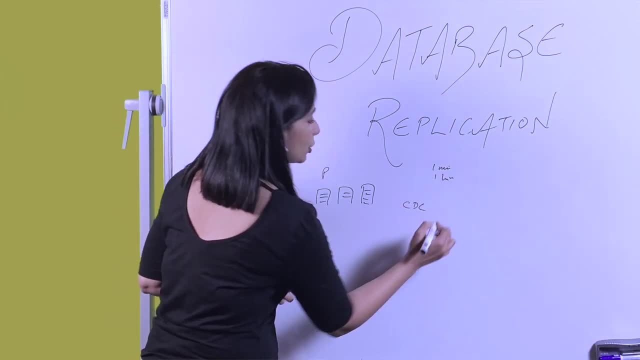 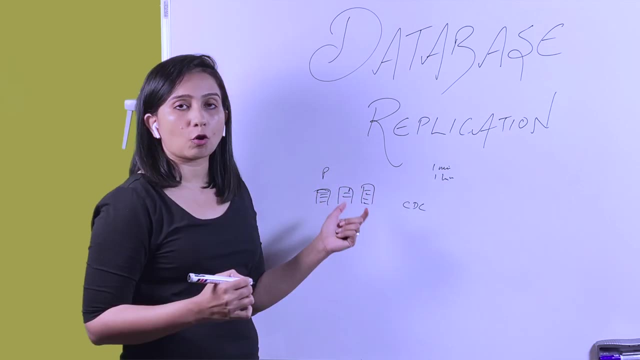 Another way is- it is sometimes also known as change data capture. In that case, what happens? even a slightest write or slightest update to one of the rows or one of the columns is captured by a running process and it is propagated to different replicas.